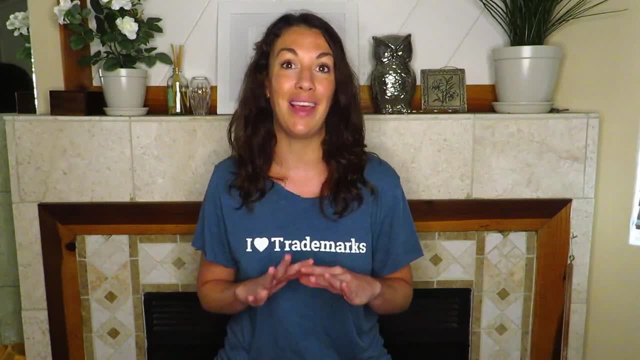 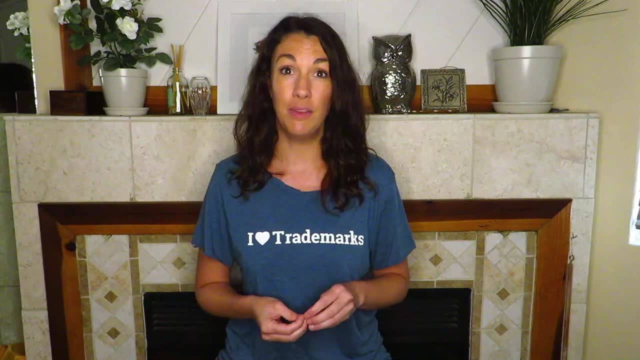 a trademark, there's a lot of things that we can mess up and that we can get wrong, And when it comes to trademark registration, you can fix some of the problems sometimes, but often there are errors or issues that we can't go back and fix in the trademark application. 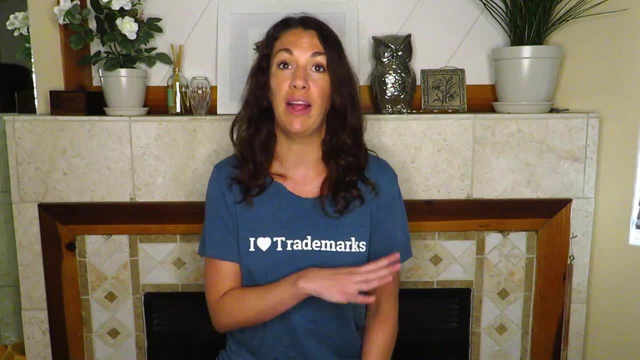 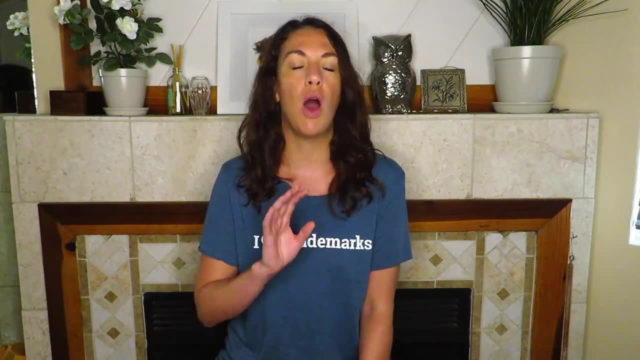 Often we have to fix them and then we have to fix them again. So I think it's important to scrap the initial one and go back and start from scratch again to correct whatever those errors are. So that's what I'm going to tell you guys about is some of those common issues that I see coming. 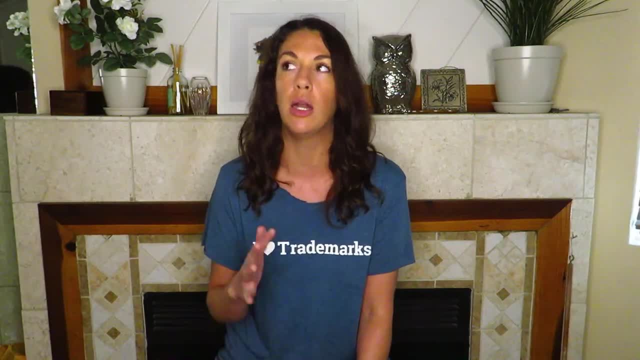 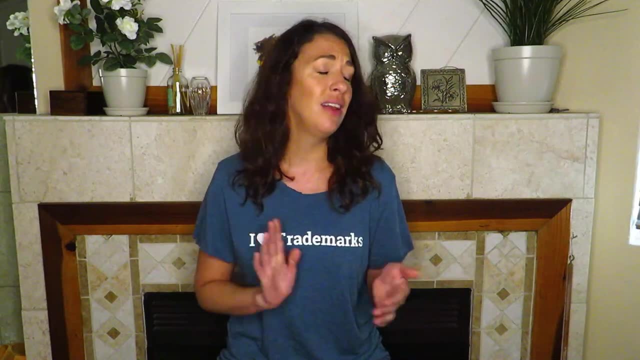 up when people try to do a trademark application and situations where it's typically going to get rejected or you're going to have some other kind of issue. The first, definitely number one thing, and I guess this doesn't really have to do with the trademark application, but the biggest mistake. 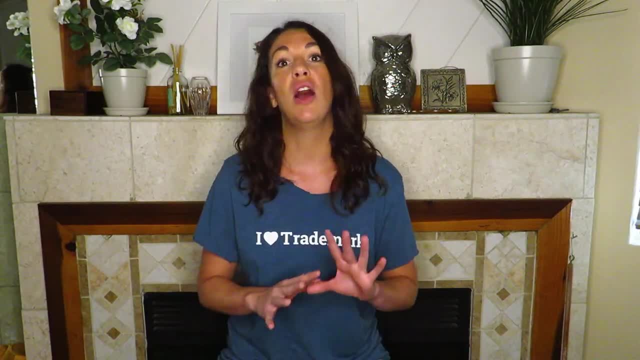 that I see in the trademark application is that you have to go back and start from scratch again. So you can't do that and it's a little bit of a plus. So I would say that the biggest mistake I see in the trademark application process is not doing a thorough enough search before you've even filed the application. 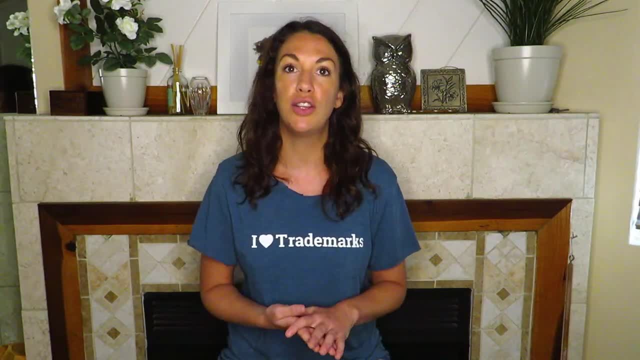 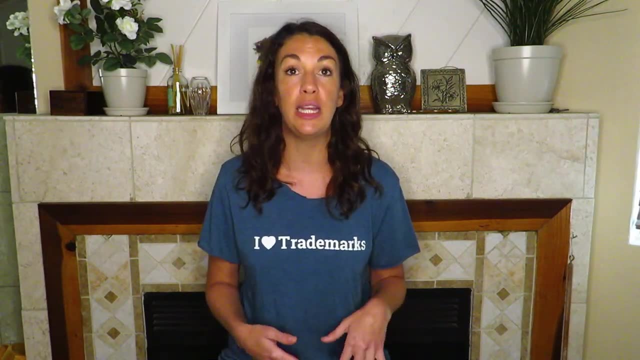 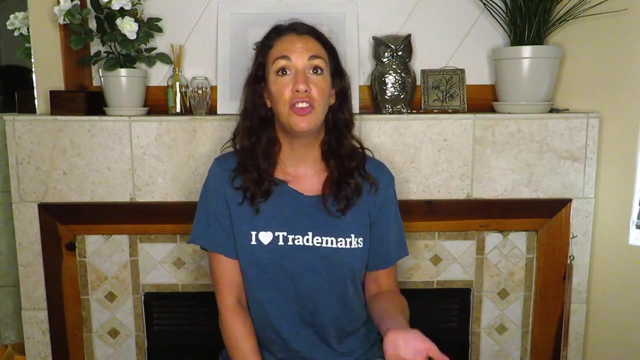 Sure, most of us know, and if you don't, you can go on to the USPTO's website and use their TESS, T-E-S-S search function to search the USPTO's database for pending and registered trademark applications. And much of the time that's what people will do: They'll go on to TESS and search. for their trademark application and they'll find that they've been able to do it. So that's a big one, And I think it's a really good thing that we've had this kind of a situation where people are not able to do it. 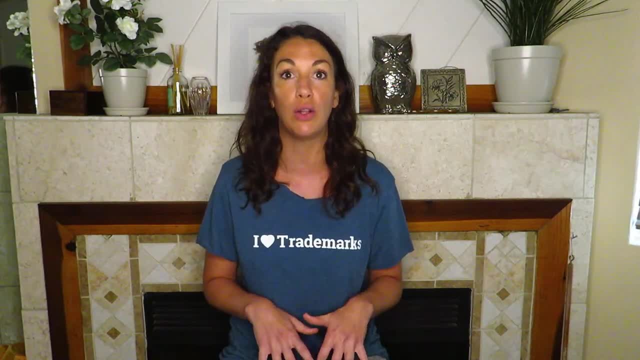 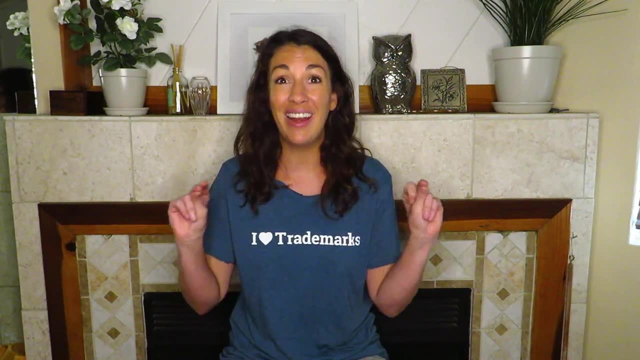 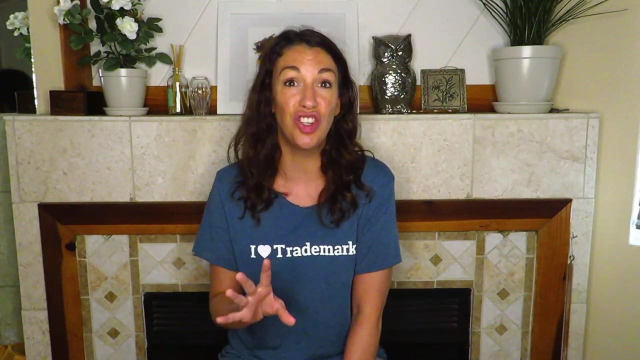 their exact business name or the exact trademark that they're looking to register, to see if something pops up- and often nothing will pop up, and so we'll think: all right, we're in the clear, ready to go. let's do this trademark thing, but that direct hit search of just looking for exactly the 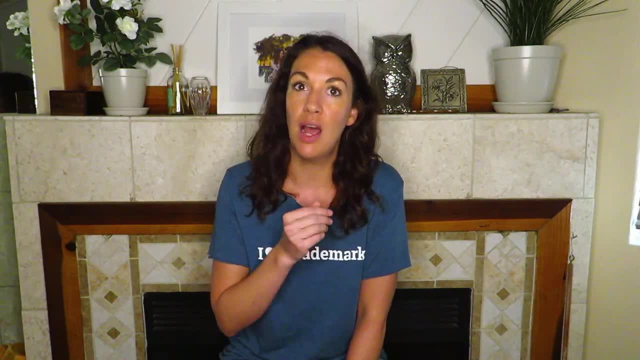 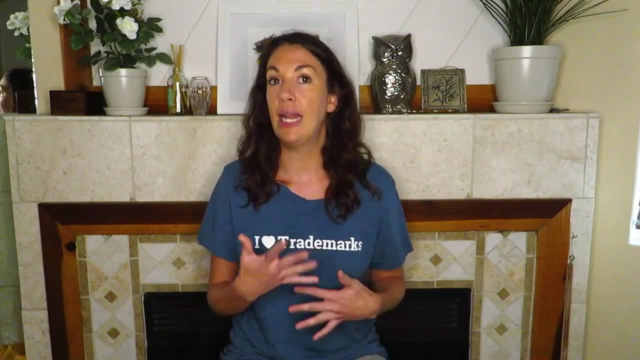 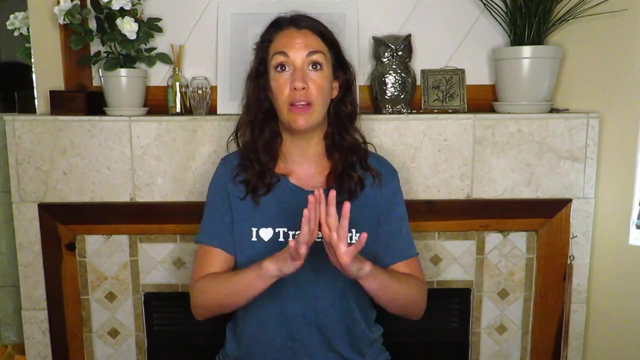 trademark that you're dealing with is, most of the time, not good enough. when we're dealing with trademarks and trademark infringement and getting a trademark registered, we need to not focus just on that exact trademark, but we need to focus on similar trademarks as well and look at potentially. 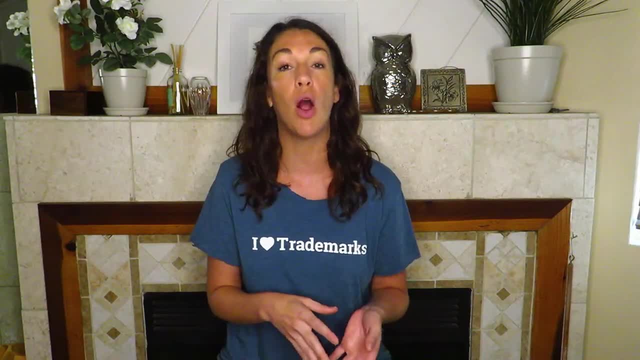 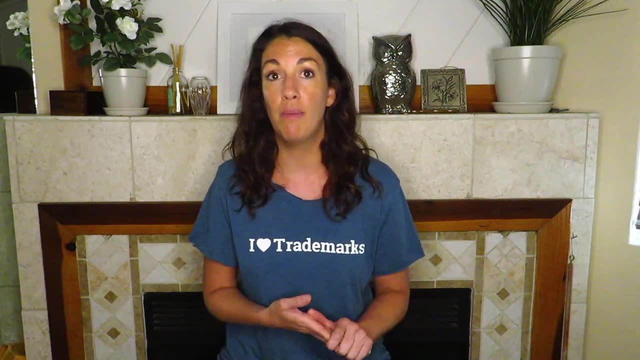 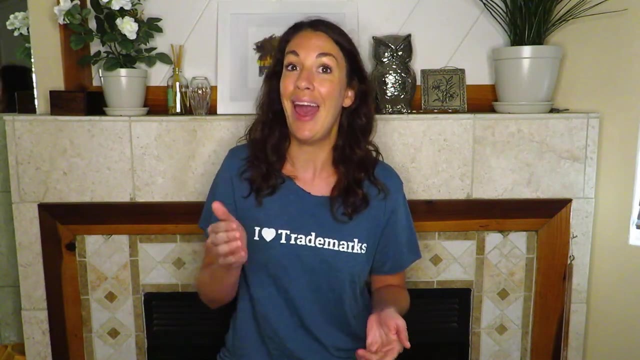 other similar trademarks that might get in the way of our trademark registration. so that means searching for different, variable spelling of your trademark. if your, if your trademark includes a word that starts with a trademark, you're looking for something that's similar to your trademark with a c- oftentimes someone will use that word- but with a k instead. searching for that, uh, alternate. 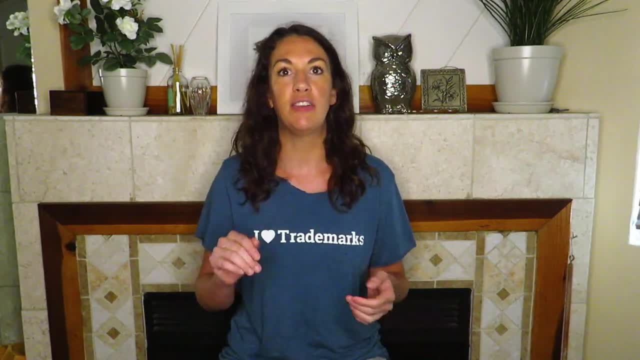 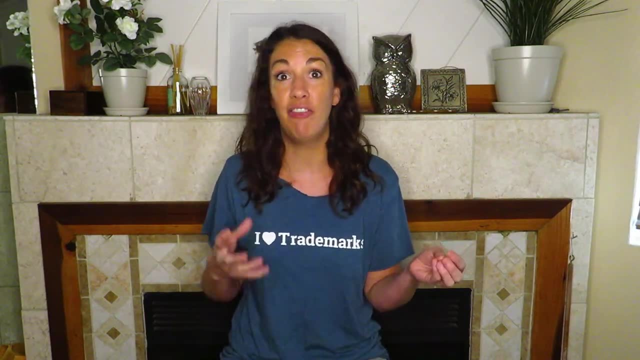 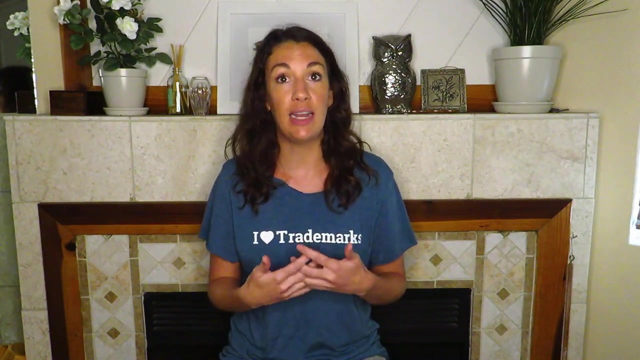 spellings: um. singular versus plural, uh, different words like, if we're dealing with dog, how about hound or pooch, or cat and feline? so any of these words, even if the trademark isn't identical, if it's similar enough, it can still impact your trademark application and your chances of getting. 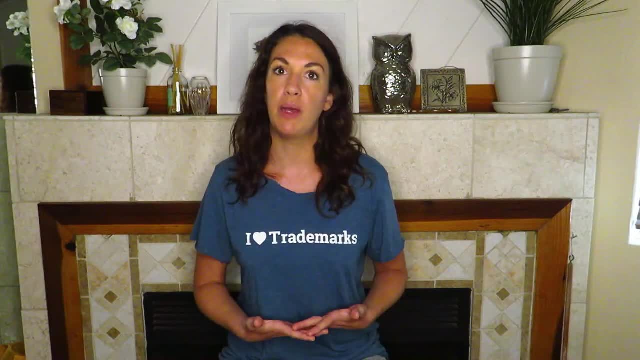 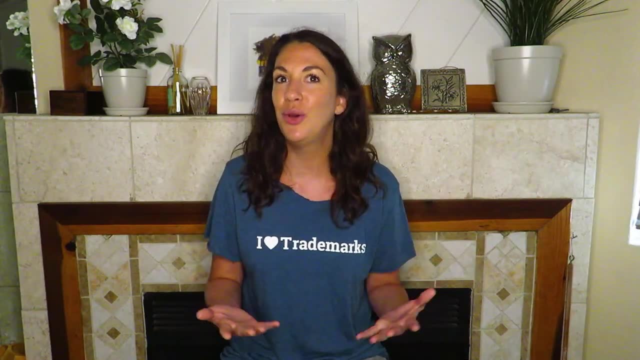 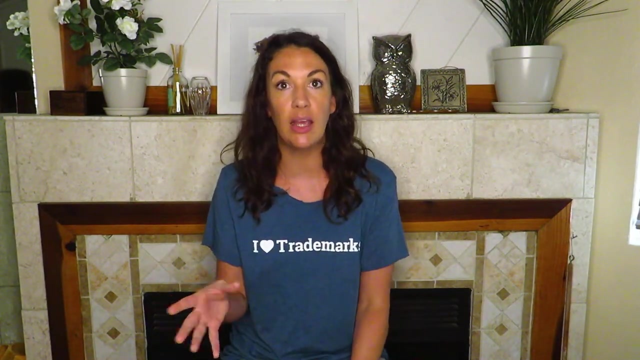 a trademark registered and so, at a bare minimum, typically we want to search the uspto's database, we want to use that test search system and we want to use a google or some other online search engine to see what else is out there just on the internet, not specifically just with the uspto registrations, and we'll also 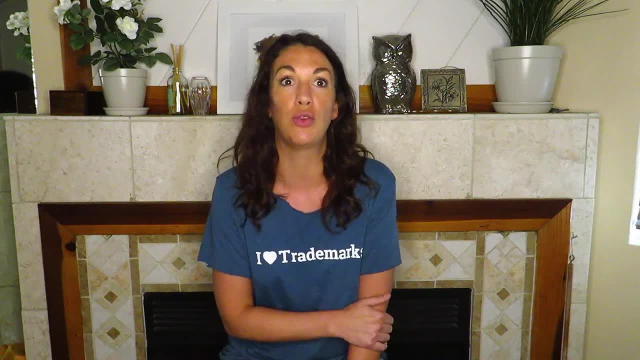 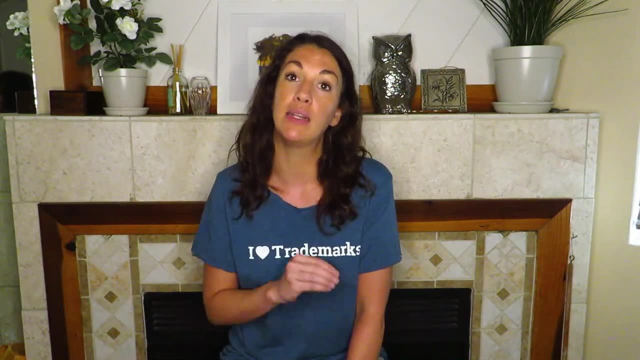 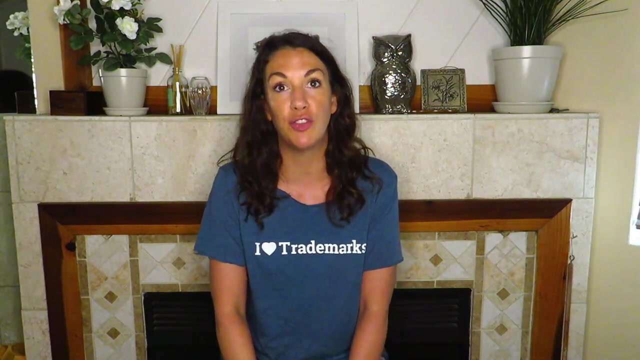 commonly want to search state level business registrations or state level trademark registrations to get a full idea of everything that's out there and we want to make sure that everything that's out there that might impact our trademark. so that's the first big mistake that i see often happening is people not doing a thorough enough search or not searching. 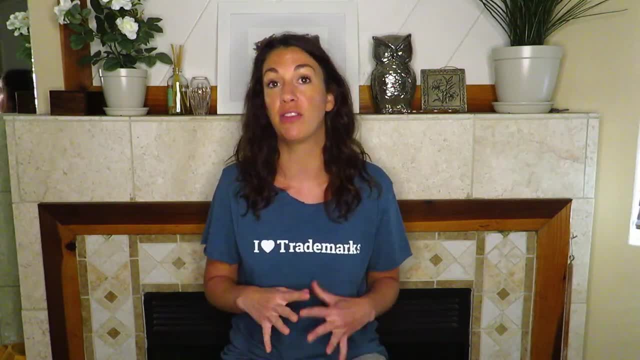 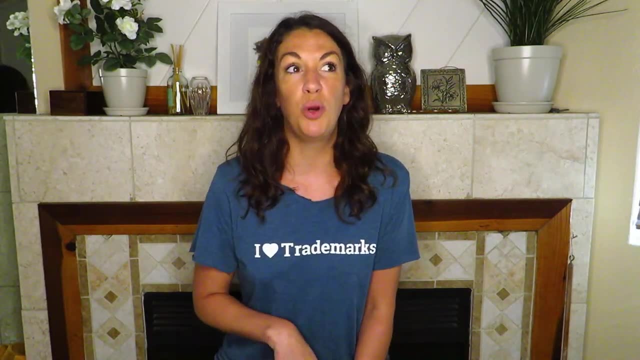 for the right types of things to see if their trademarks even going to be available and able to be registered. so the second mistake that i see come up quite often is putting the wrong trademark on the drawing, on the application. so on the trademark application there's going to be a spot. 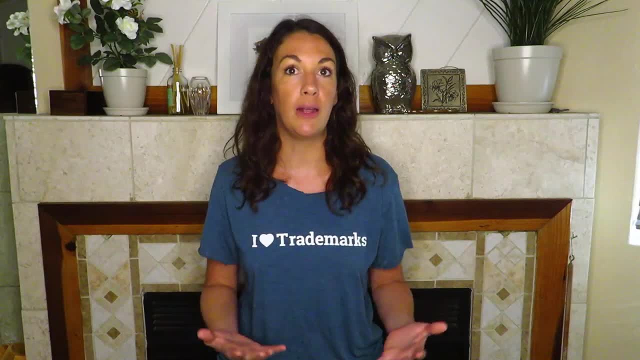 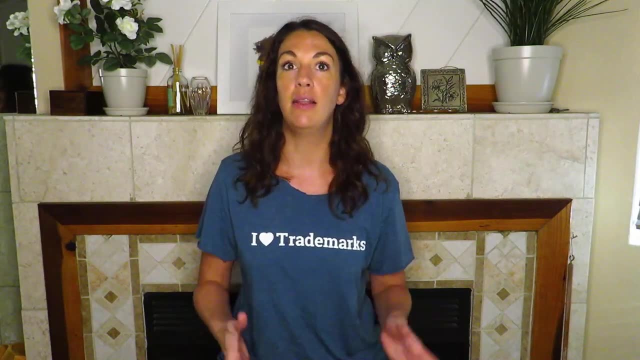 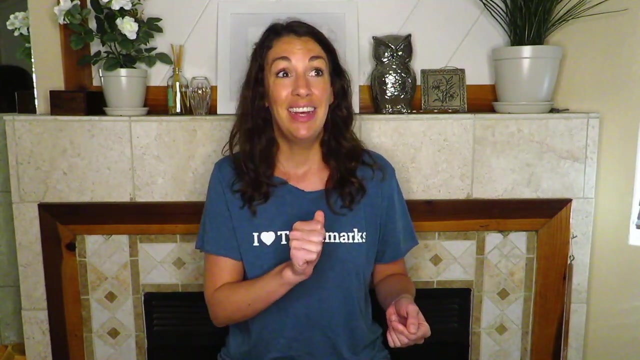 on the drawing of the mark which, if we're dealing with just standard characters, it's just going to be the words in your trademark, or if we're doing a logo or some kind of a design, then it's going to be the logo, whatever it is that we're trying to trademark. that's the drawing, but often what is? 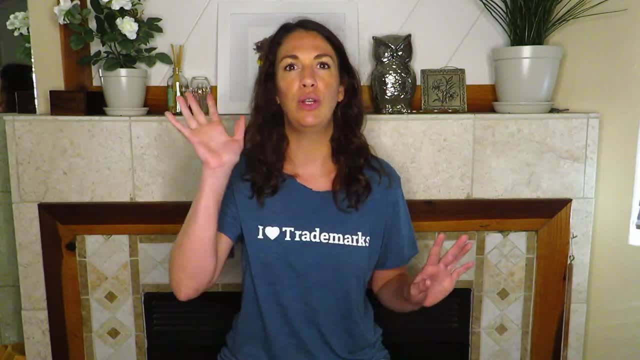 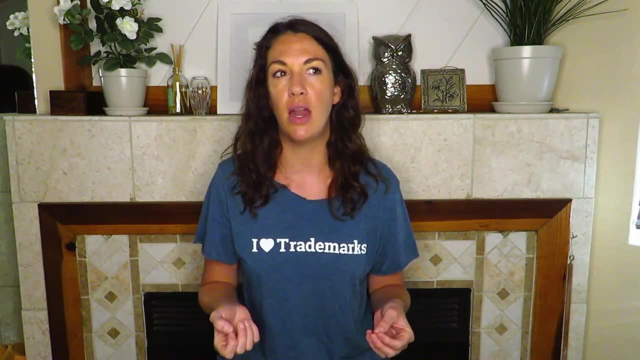 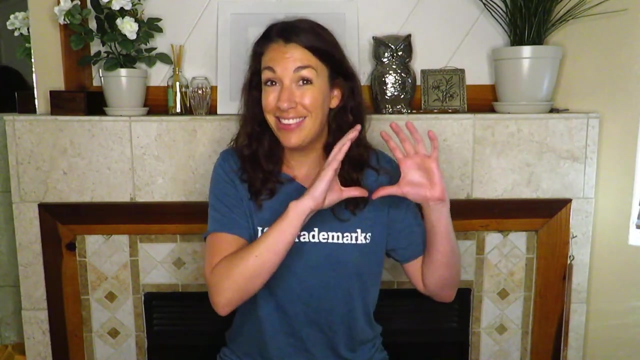 uploaded or provided, as the drawing isn't actually the trademark that it's going to be, and so commonly this comes up with logos a lot more often than standard characters. but so let's say we've got a logo that we want to register the trademark for. exactly how we provide that logo on the application needs to be how we're going to. 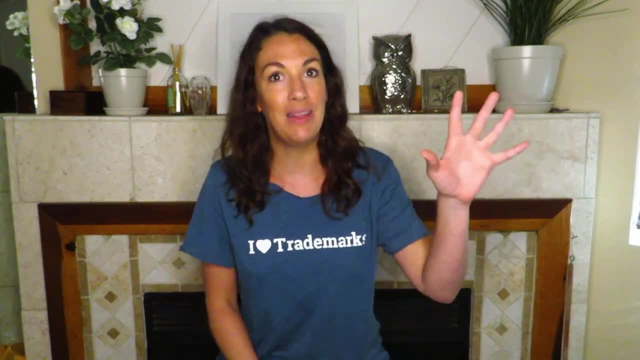 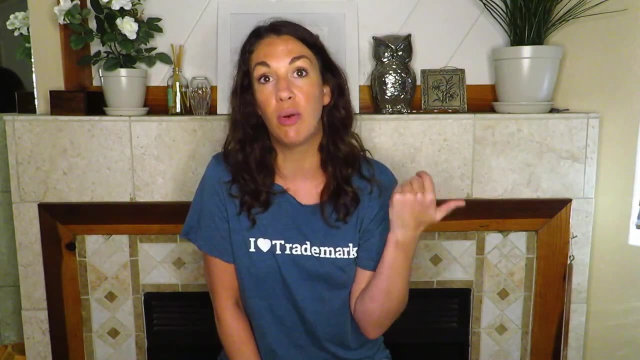 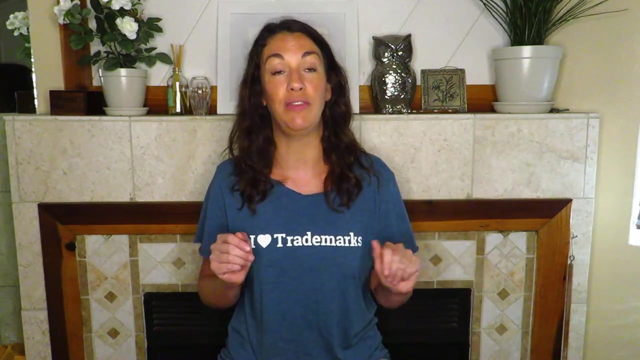 actually use it as a trademark. so we can't submit the application with this logo and then change it and then what we actually end up using is different from what we identified on the application. they need to match the trademark as we're actually using it and as we. 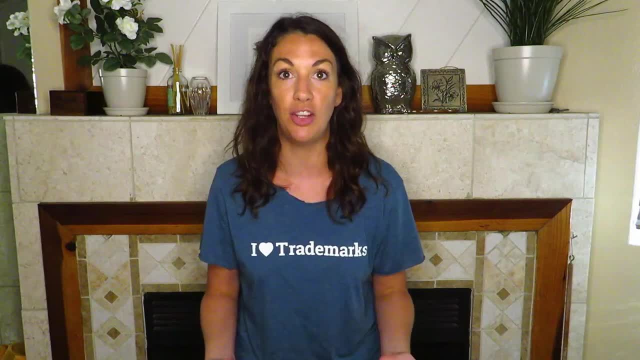 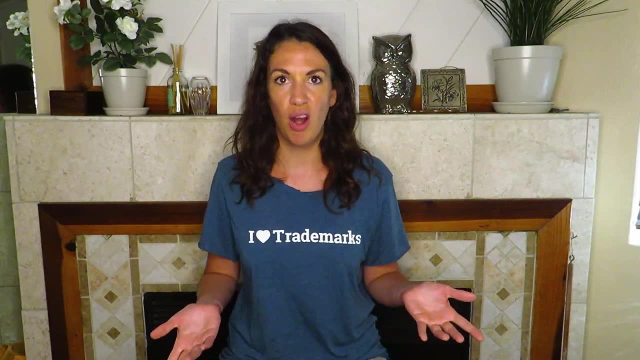 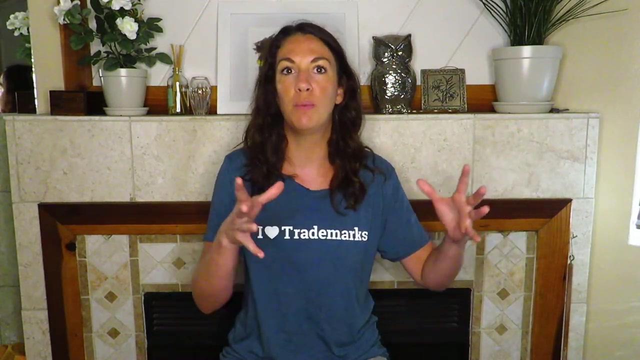 identified it or designated it on the application needs to match, or if we are um- you know, dealing with standard character marks- if we put our drawing of the trademark with um, let's say three words, but it's all. we've combined them all into one word so we don't have 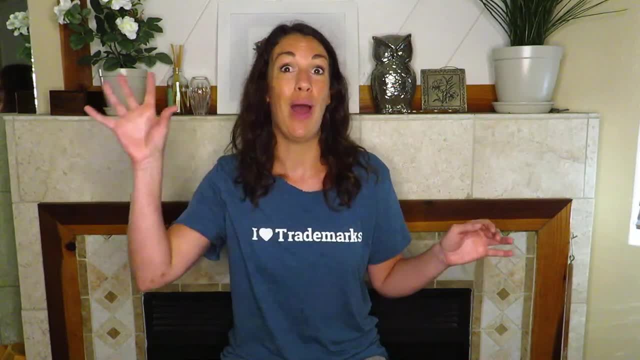 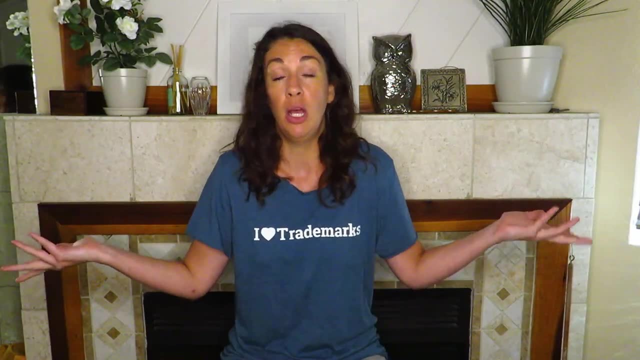 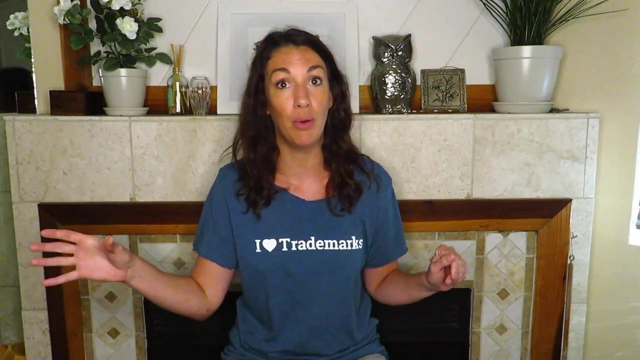 spaces in between, it's all one word, but then, as we're actually using it, if we do separate it out, that's a different trademark. um, i mean, for the most part it's it's not the same and it's not going to be considered the same if we're using it as three separate words. but on the application, 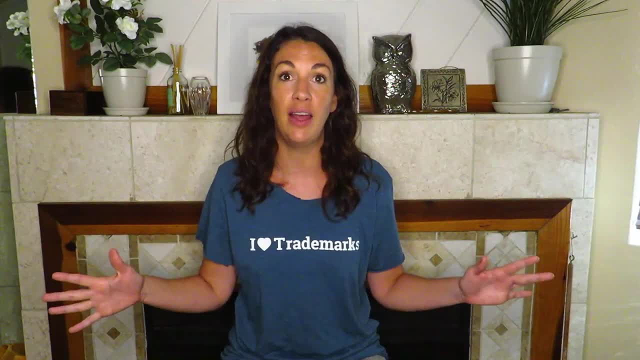 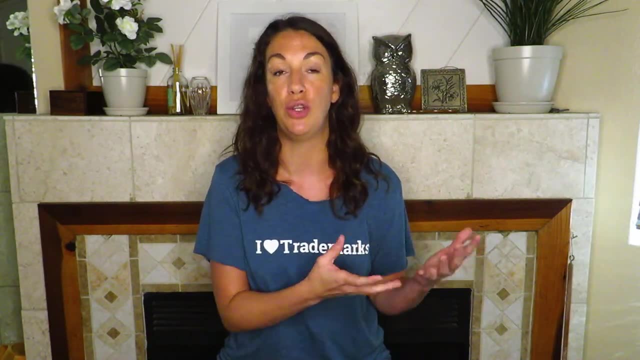 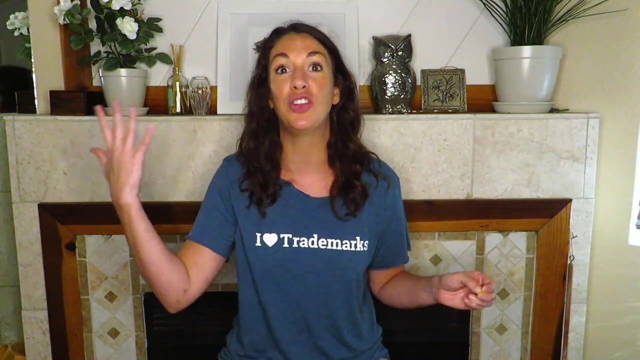 we've identified it as one word that's not going to fly. so that's a big mistake that i see come up quite often is not putting the trademark as we're going to use it as the drawing or or making one um trademark or submitting something, but then we're actually using it in a different way or a. 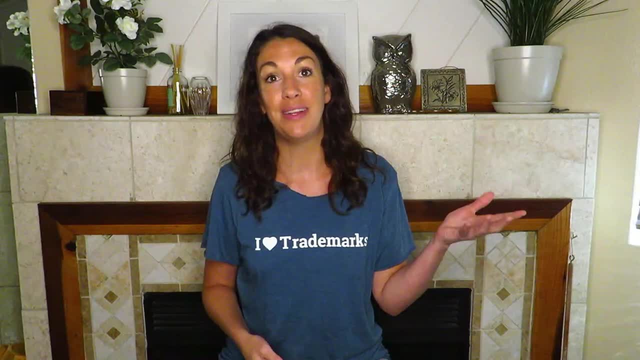 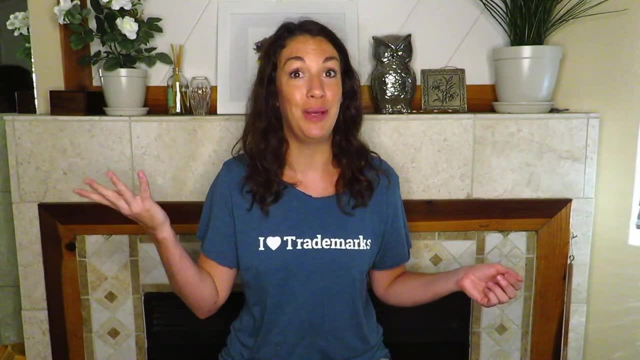 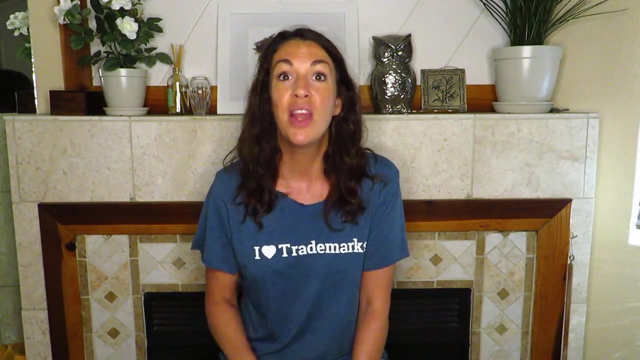 different way than what we're actually using. but the point is that the trademark is the trademark or trademark as we've identified it on. the application needs to match exactly how you actually use it. which brings me to my fourth mistake that i commonly see popping up is submitting improper specimens. so now, when i say the mark as we've identified it on the 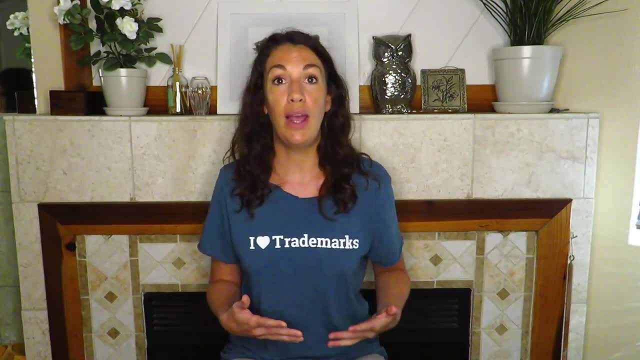 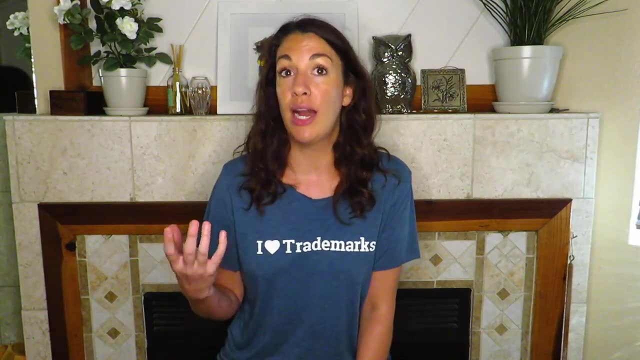 application needs to match how we're actually using it. the way that the trademark office sees how we're using it is with this specimen: trademark is the trademark that we're using. it is the file. So we are going to have to submit to the USPTO proof of us using the trademark in commerce. 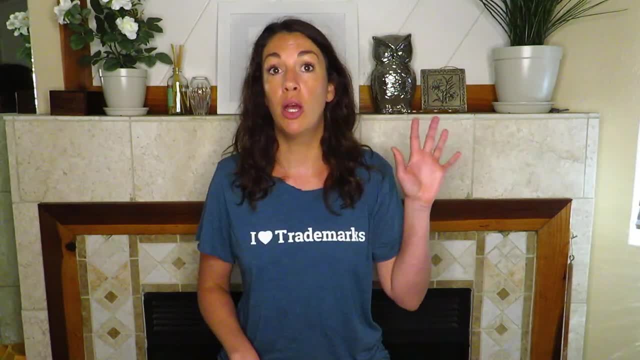 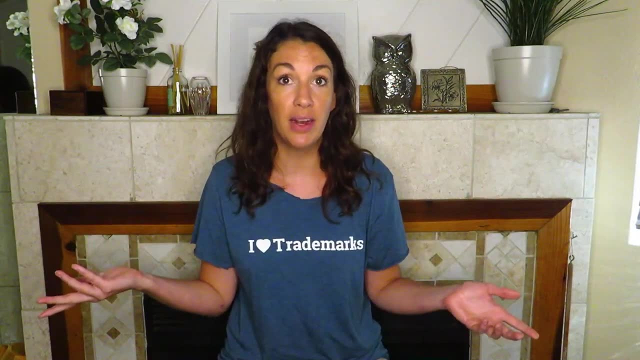 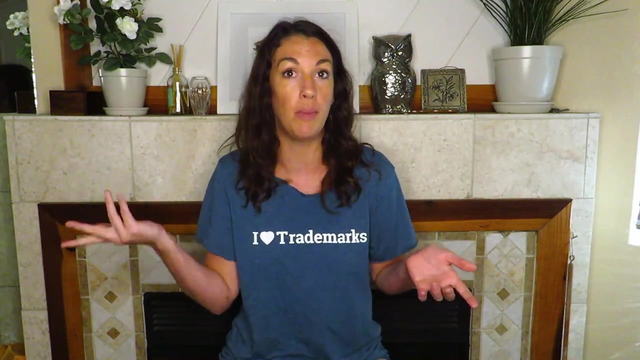 and that's what this specimen is, And so if the mark on the application doesn't exactly match the mark on the drawing, then the specimen is going to be rejected. It doesn't actually show you using this trademark in commerce. It shows you using some other kind of similar trademark, but not the 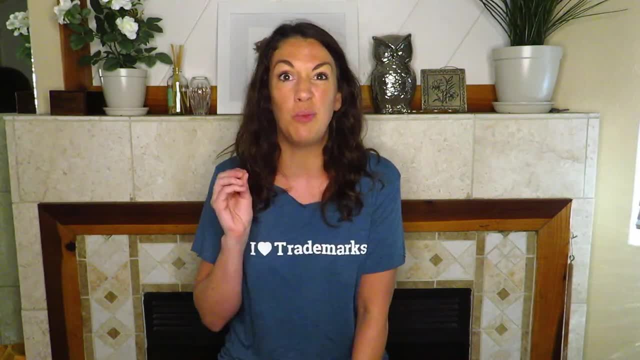 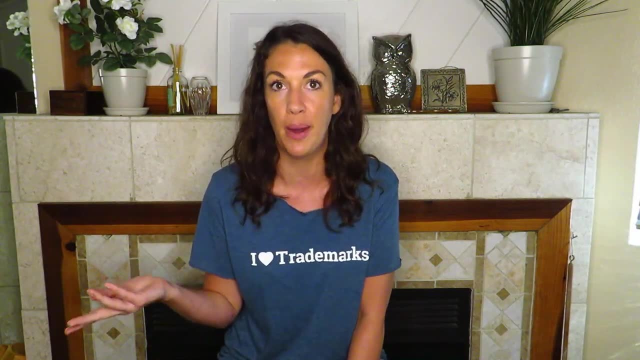 one that you applied for. Another big mistake that I see is people just uploading, especially with logos. again, people just uploading another picture of the logo as the specimen. That's not, that's not right. That's not what the specimen is supposed to be. The drawing you would upload just 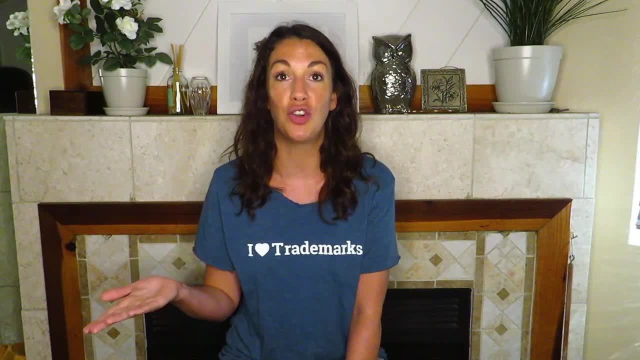 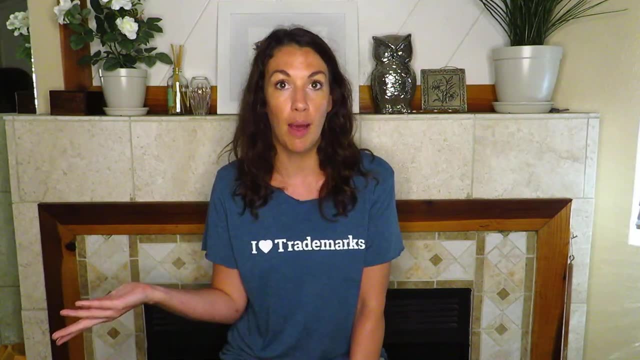 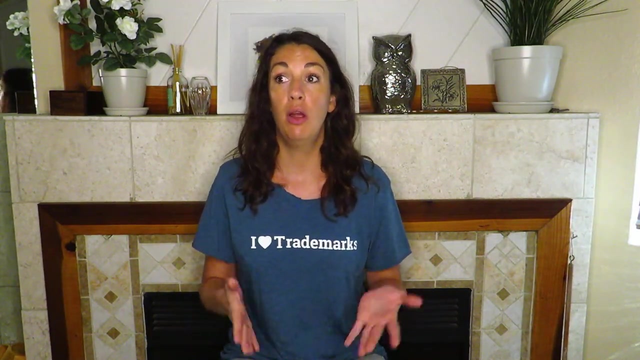 an image file of the logo, but the specimen needs to demonstrate that the logo is being used in connection with the goods and services that you've identified on the trademark application, And so it's important Be careful when we're preparing the specimen files, making sure the trademark as we've got it on the 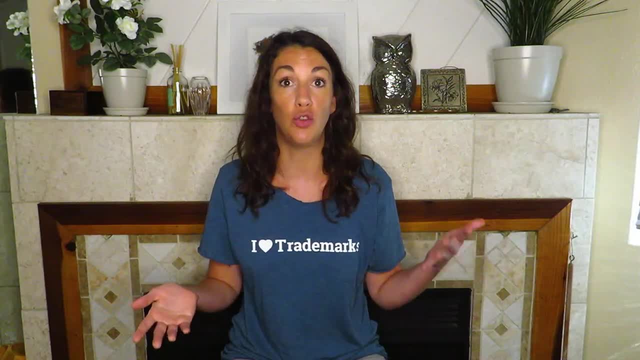 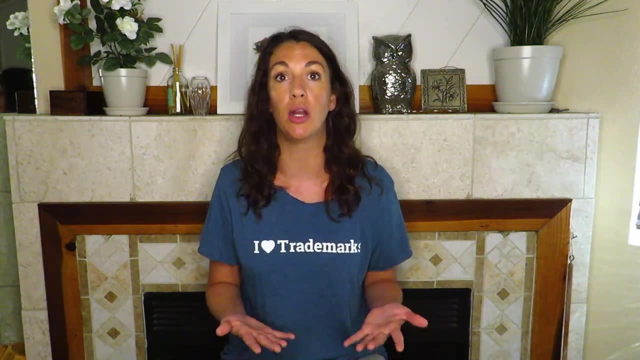 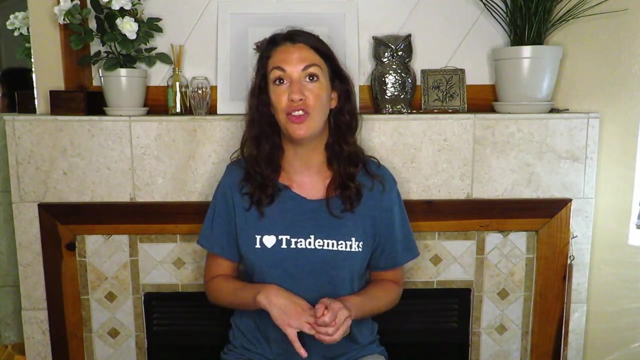 specimen actually matches the trademark as it was in the drawing on the application and that the specimen actually shows use of the trademark in commerce. Another really common mistake or error that I see on trademark applications has to do with the goods and services that are gonna be on. 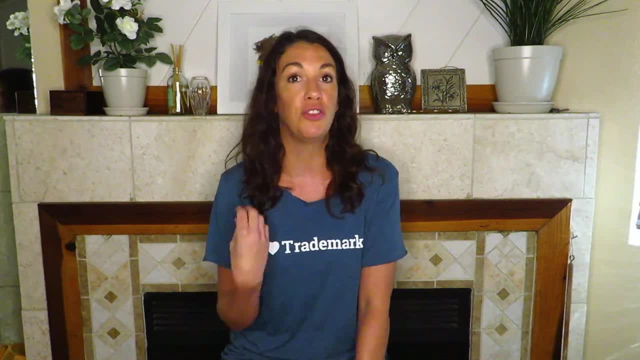 the trademark application. So I'm going to be using the trademark application as a reference to the trademark application. So I'm going to be using the trademark application as a reference to the trademark application or on the registration. So when we're submitting an application for 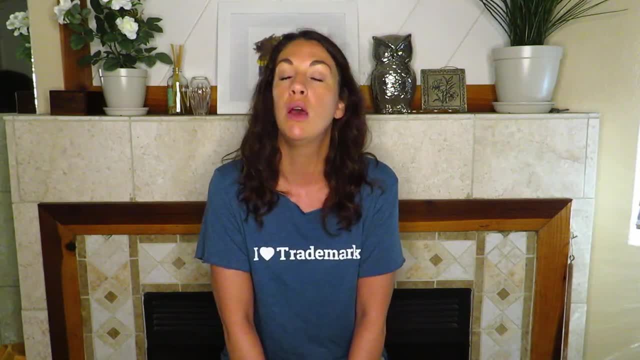 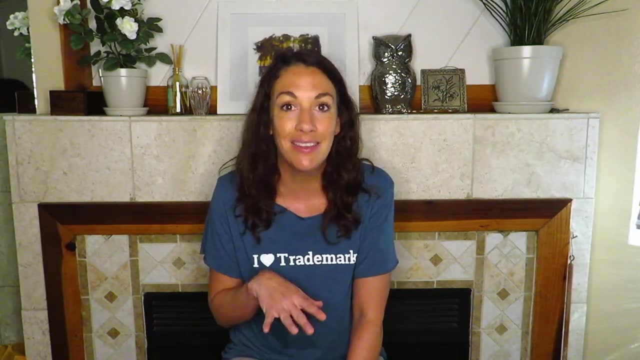 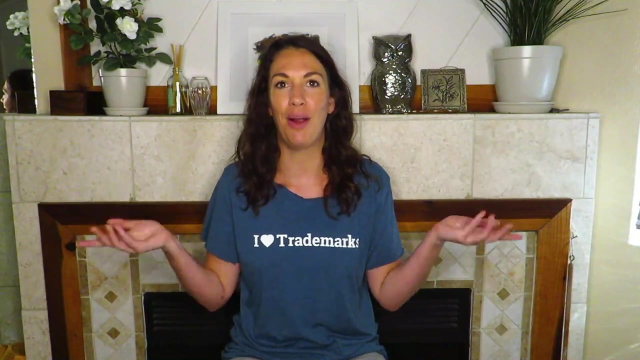 registering a trademark, we have to be specific as to the goods and services that the trademark is going to be used in connection with, And there are 45 different classes of goods and services and each class is broken up into, I mean, an infinite number of different descriptions or kind of 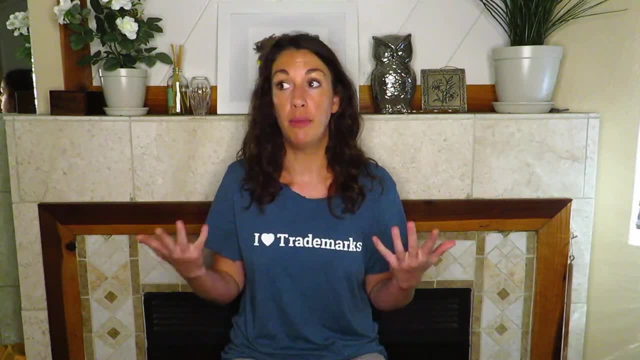 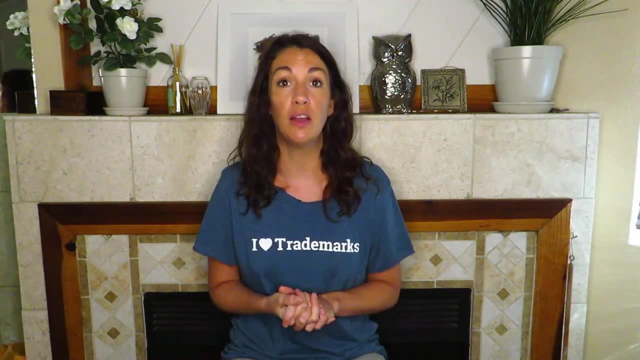 different categories within each class, And now some of these classes are very, very different, But the others are very specific. So, let's say, we're selling shoes, we can get caught up in plants. So, let's say we're selling shoes, we can get super specific what the types of shoes were selling and 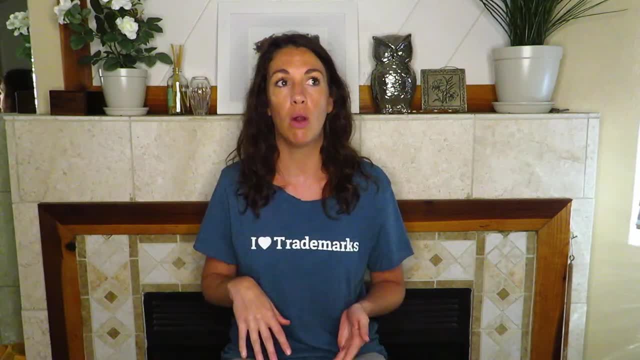 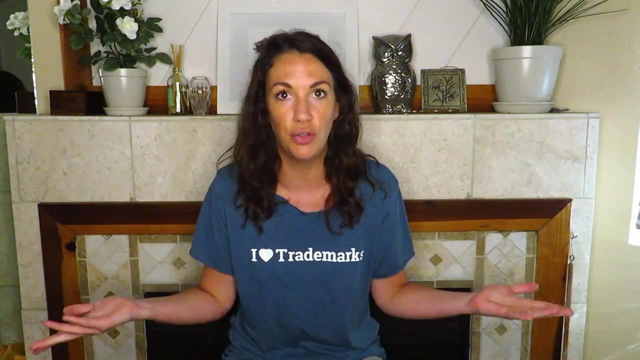 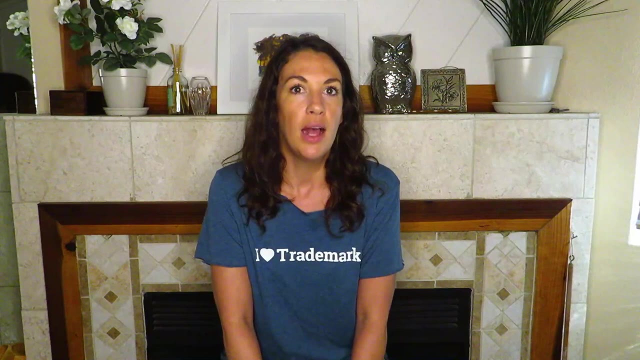 identify that on the application. we can say we're selling sandals or we're selling high heels or platform tennis shoes or form tennis shoes or sport shoes, basketball shoes. we can be very specific Or we can be very broad. we can say we're selling footwear or shoes And so we have options here of 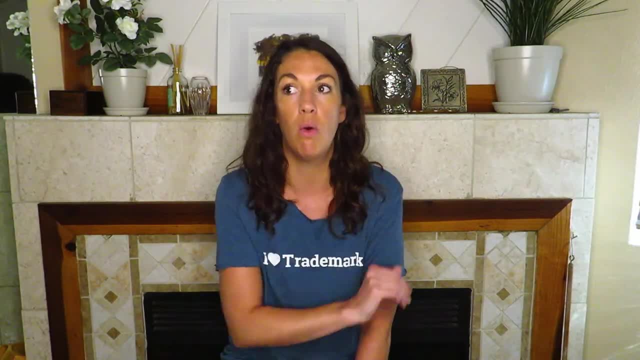 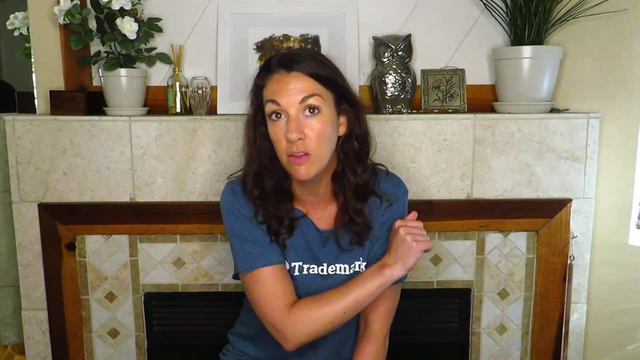 And so we have options here of being thick and thin, not thin, So again with something that is low, in being very specific or being very broad, And sometimes we wanna fall somewhere in the middle, but sometimes we wanna be very specific. This kind of goes back to that clearance search. 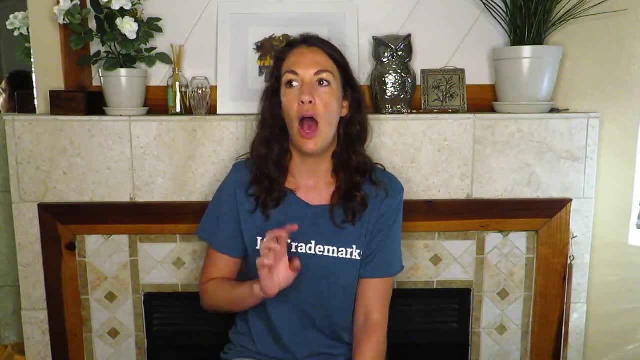 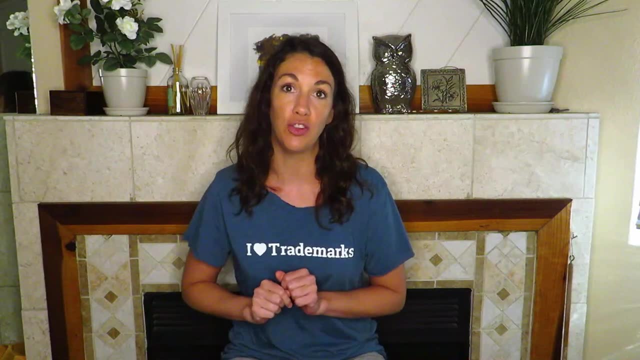 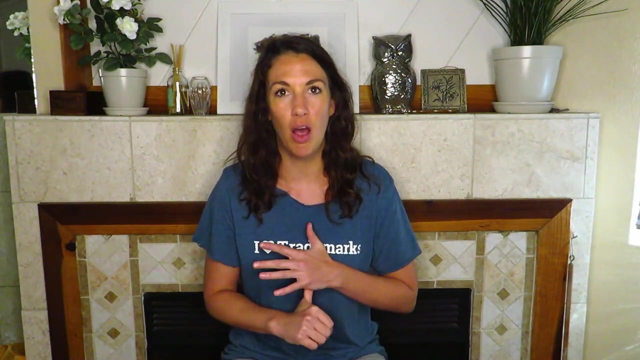 and the searching part that I talked about, because that helps in a lot of cases figure out what strategy we need to take with the goods and services descriptions too. But so with these goods and services and the proper classes on the application- a big mistake that I commonly see. 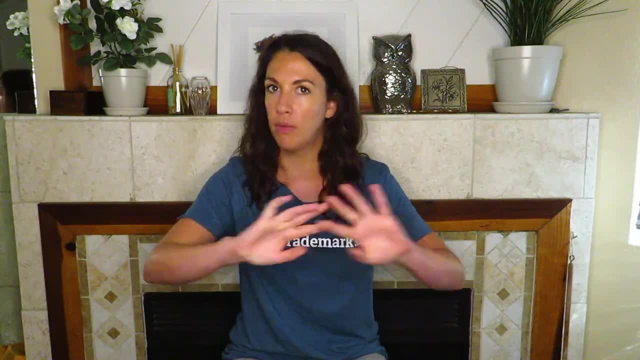 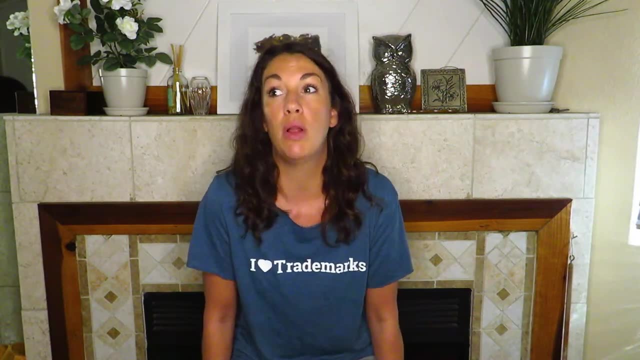 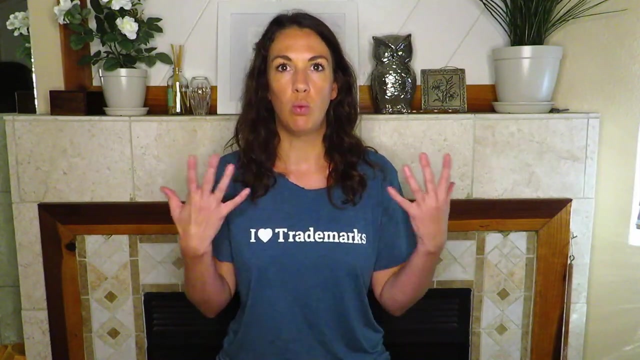 is just getting flat out the wrong class altogether, just doing something completely unrelated. So let's say often, for example, if you are starting an online boutique like a clothing boutique, and that's what you're providing, is this website where people can buy clothes? 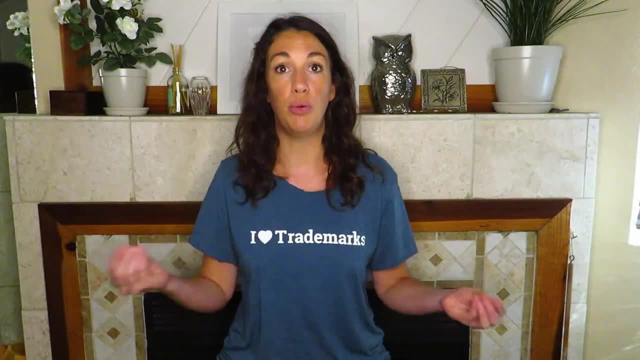 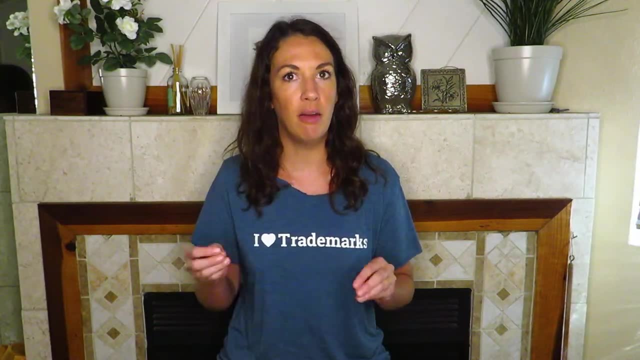 If you're not actually making the clothes yourselves. let's say it's a boutique, so you have other brands in your store that you're gonna be selling. On the trademark application, you wanna be careful and think about what is the service or the good I'm providing. 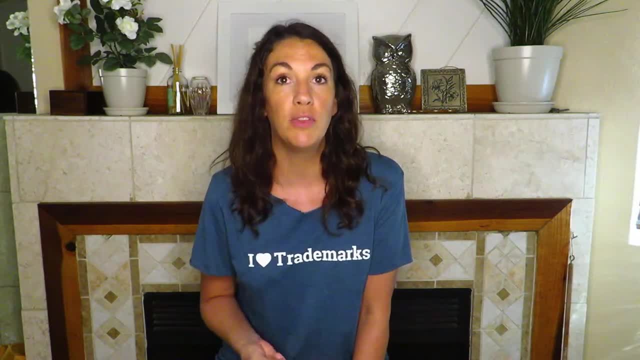 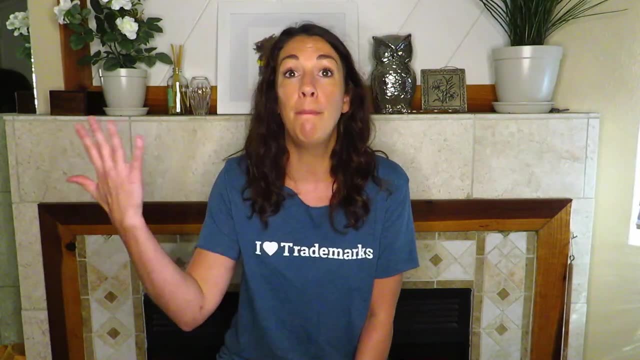 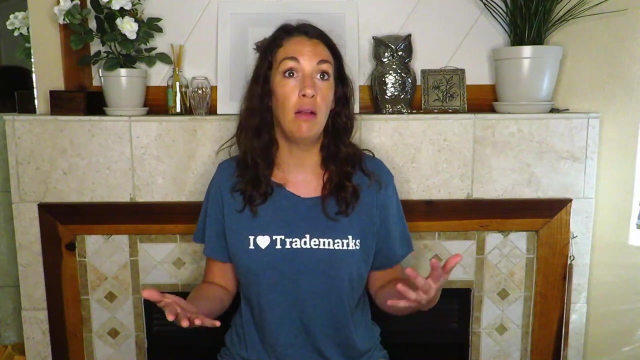 You aren't actually providing those clothing items. You're not producing the shirts or the dresses or the clothes. The other company's brand, your brand, doesn't appear on those products. What you're providing is this website, this retail, online shopping website that sells the brands of others. 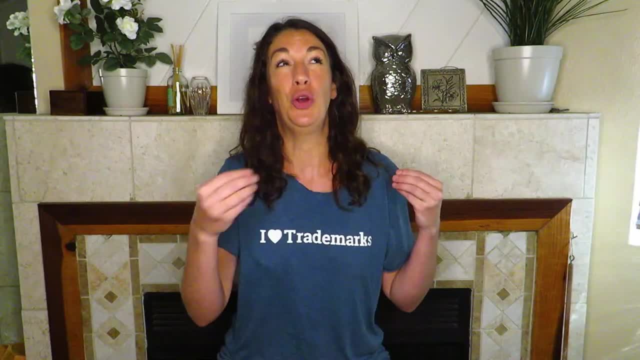 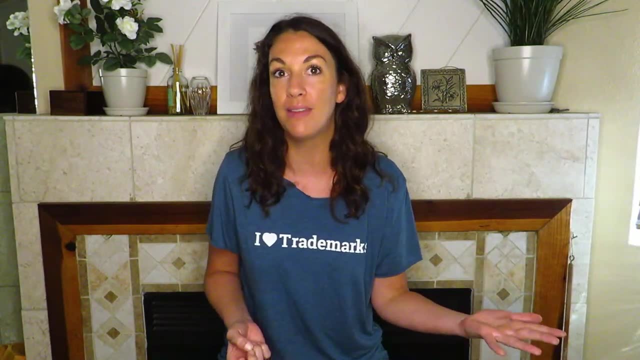 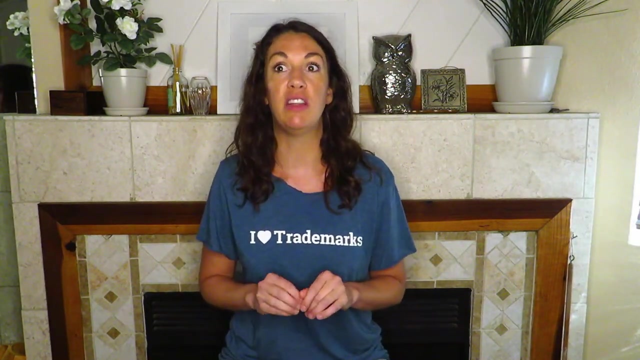 And so it's often that differentiation of the goods that I'm selling versus what I'm actually providing, which is the website or the service of the website, that people commonly get mixed up, And those goods and service descriptions are often going to be difficult to correct. 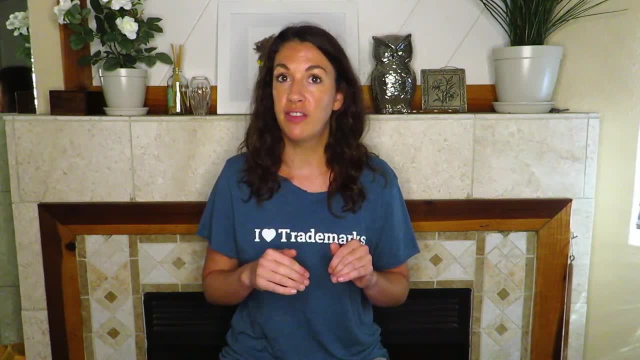 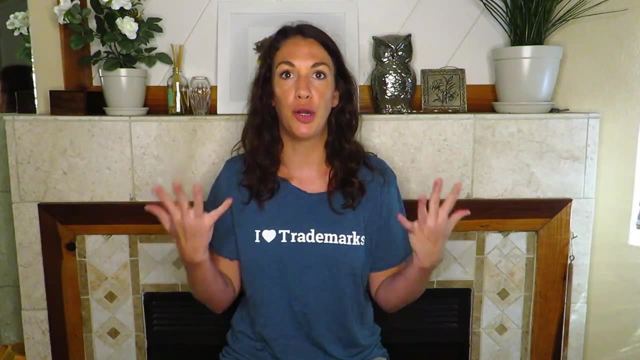 So we can, in most cases, change our goods and services descriptions to be more narrow or to be more specific, but we can't change them to be broader. So if there is some kind of an issue with your goods and services after you've submitted your application, 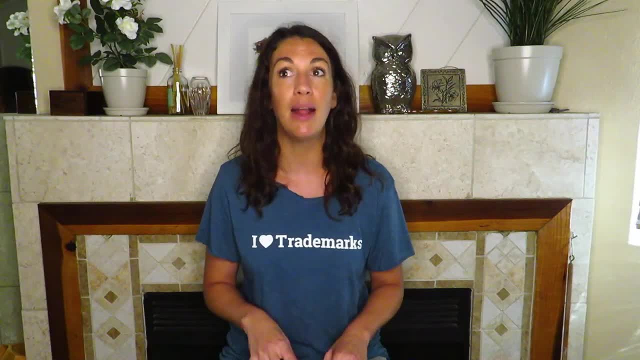 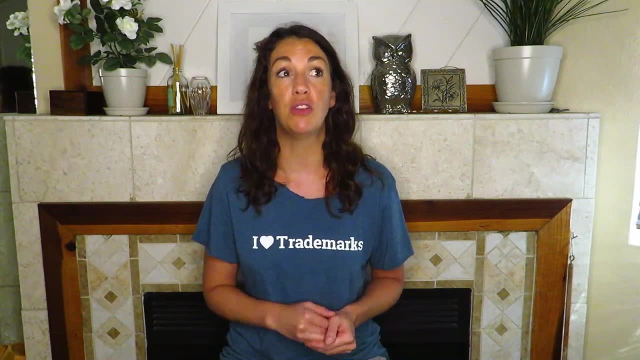 there might be an opportunity to correct it and to fix it, but there might not. So it's important that we know what route we're taking with the goods and services descriptions before we file the application, because we don't wanna risk getting it wrong. 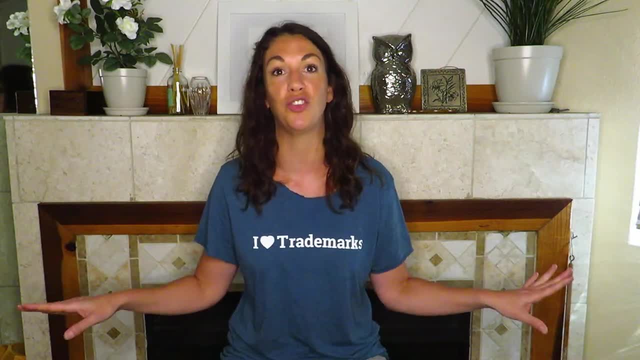 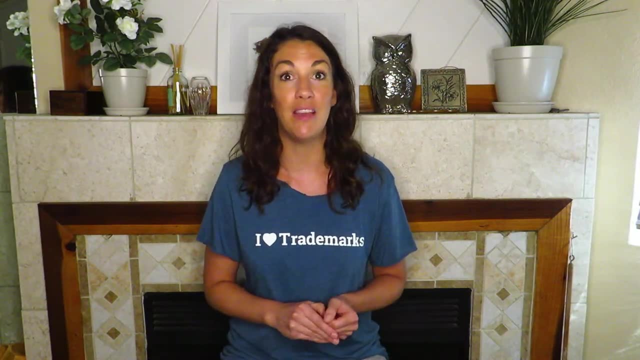 or doing it in some way that can damage the whole rest of the registration process. Another big mistake that I see that it's tough because it often doesn't come to light until far later on, after the trademark's already registered- but a big mistake that I see. 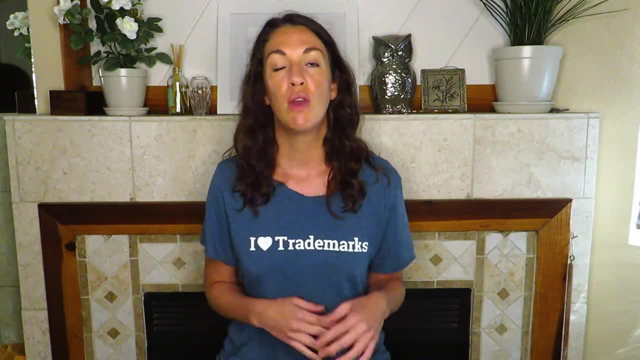 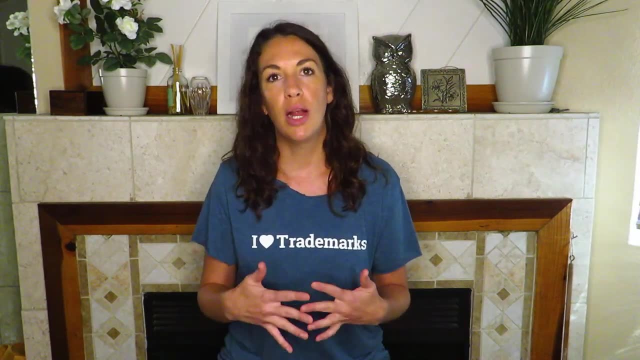 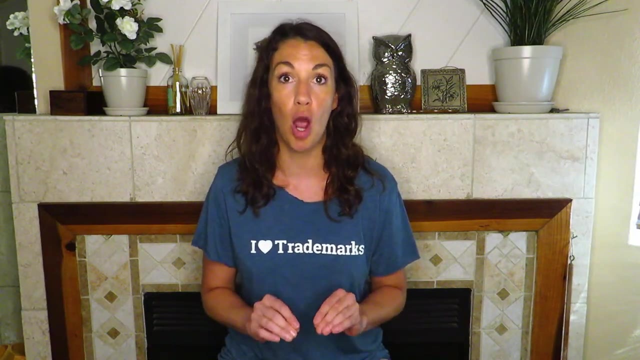 is using the wrong dates of first use. So, on the application, depending on the basis of filing and all that, this sometimes is different, but we're gonna have to identify the dates of first use of the trademark when we first started using the trademark in commerce. 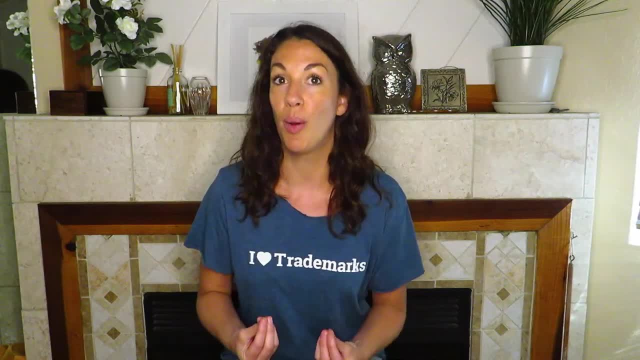 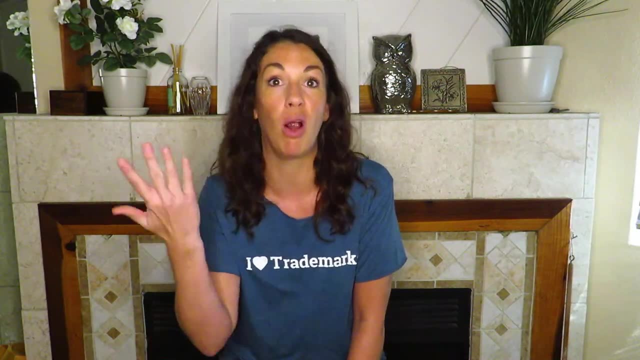 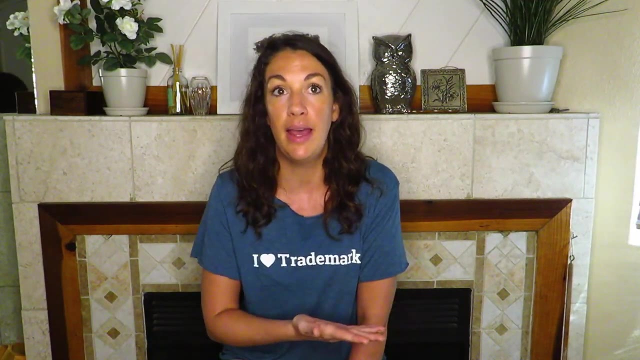 This date is when you first started using the trademark in commerce. This is not the date when you formed your LLC or the date when you bought the domain name for your business, which includes the trademark. That's not using the trademark in commerce. Forming an LLC isn't using your trademark. 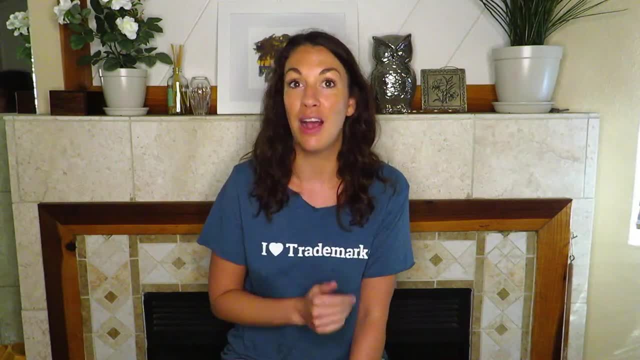 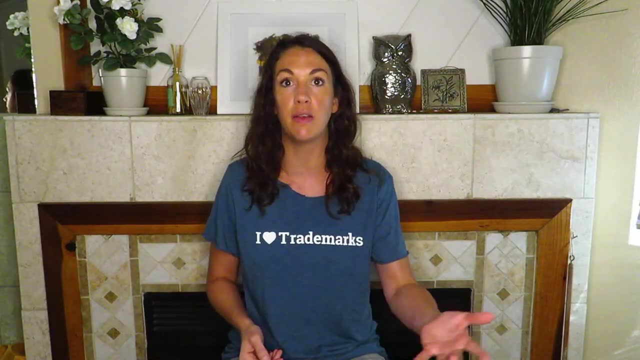 It's just forming an LLC, And so the date that we're supposed to actually put there is the date when we started using the trademark in commerce, meaning selling our products, selling our services and all of that. That's the date that we use. 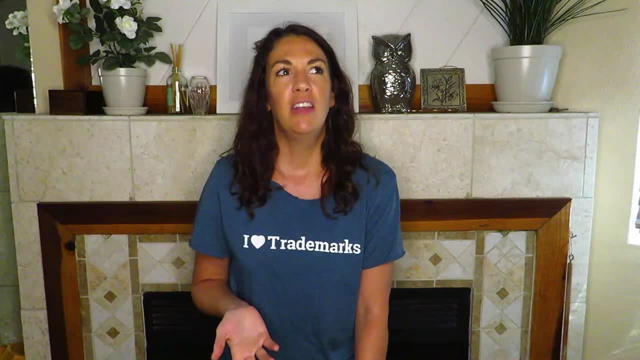 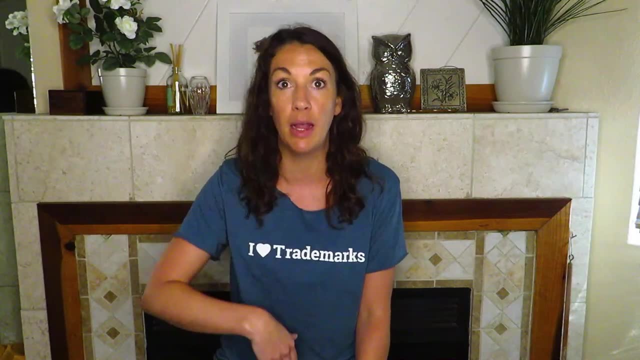 And now the reason I say that this often doesn't come up until later is because in the application process, the examining attorney, the attorney with the USPTO, who's gonna be examining your application and doing this whole thing, they're not really verifying those dates of first use. 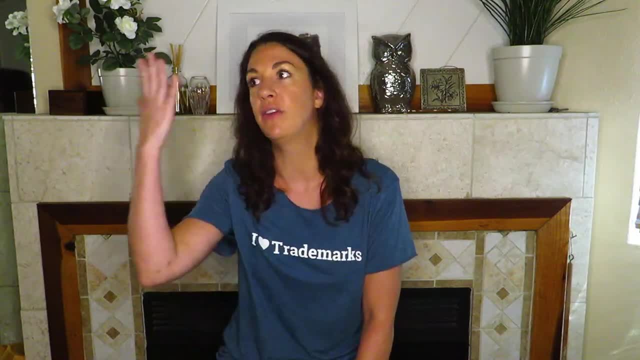 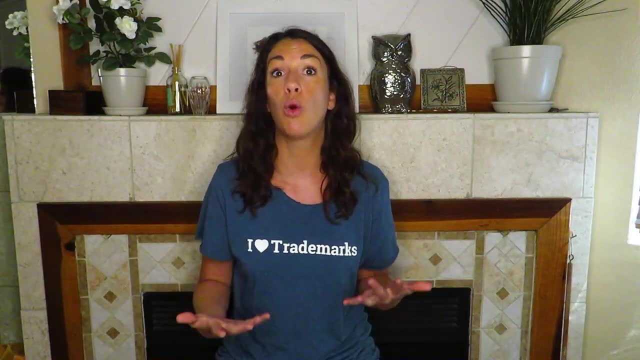 They're not gonna cross-check the date that you put and see if it corresponds with- I don't know- the date on your website. They're not checking that. They're taking our word for it Because we're promising that all the information 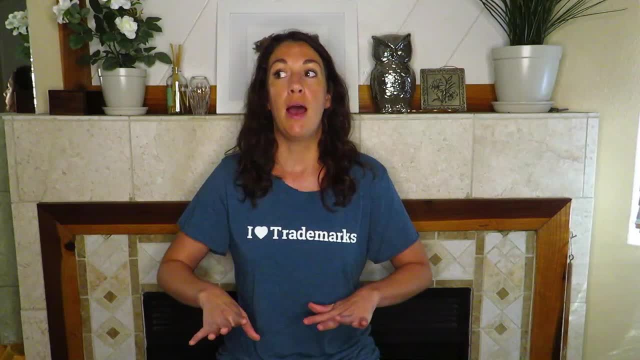 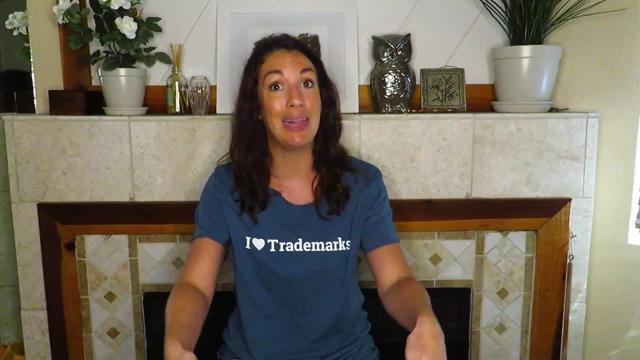 is accurate and correct. So they're taking our word for it And so whatever date we put is the date that's gonna be associated with our trademark registration. But later on down the line, if an issue comes up, let's say there's a trademark infringement issue. 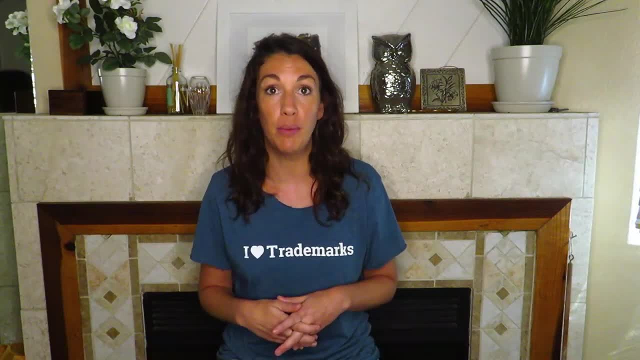 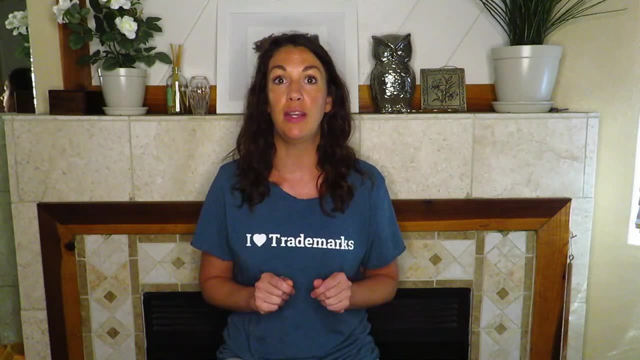 of somebody else using something similar to your trademark. that date of first use is gonna be one of the most, if not the most, important factor, Because usually it's going to be whoever used it. whoever used the trademark in Commerce first is gonna have the higher, stronger rights. 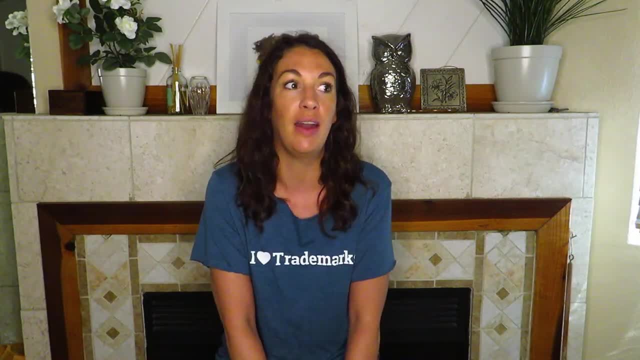 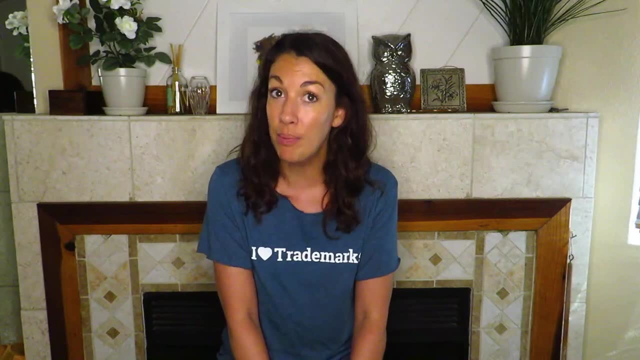 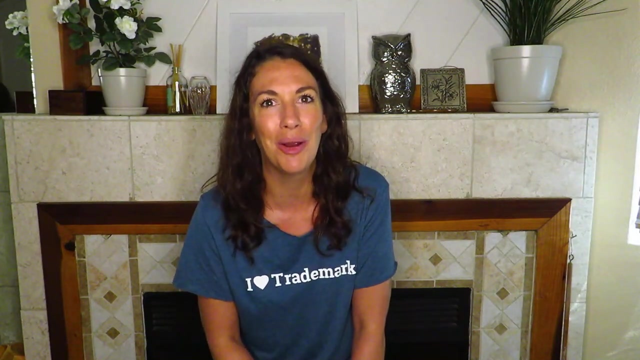 in the trademark And so if you put on your application that you started using the trademark January 1st because that's when you filed your LLC paperwork, when you go to prove that to the other party, they're gonna say no, you didn't start using your trademark then. 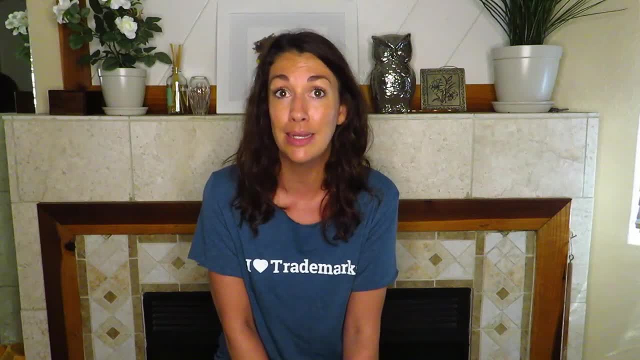 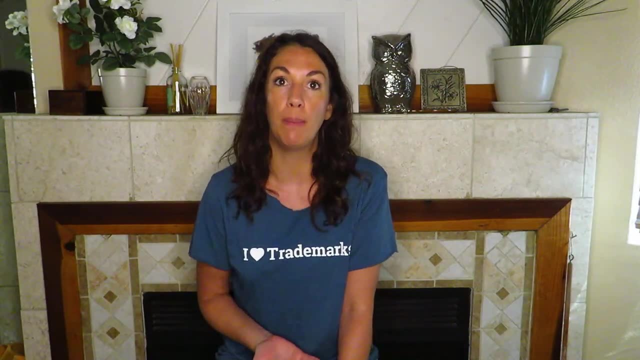 You formed your LLC on that day, but you did not start using your trademark that day, And so that's gonna, kind of you know, start to feel a little bit damage your side, and from that can potentially come some other issues. because now it's come to, 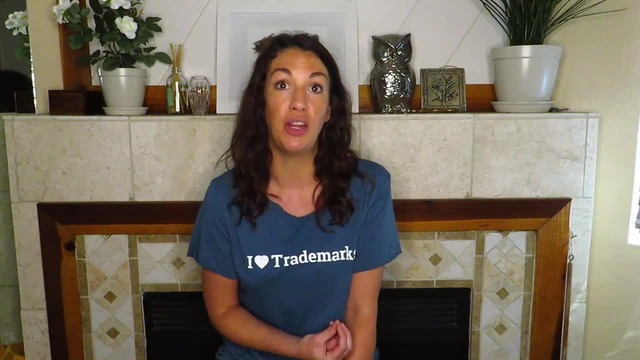 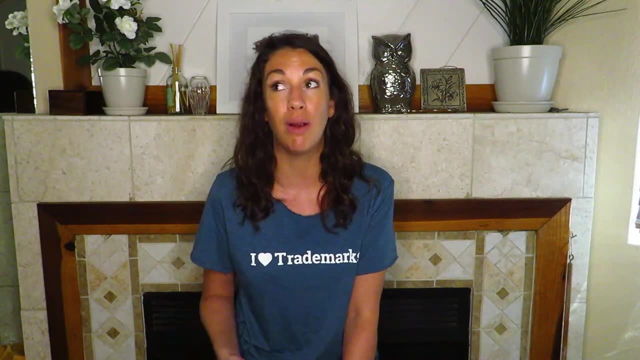 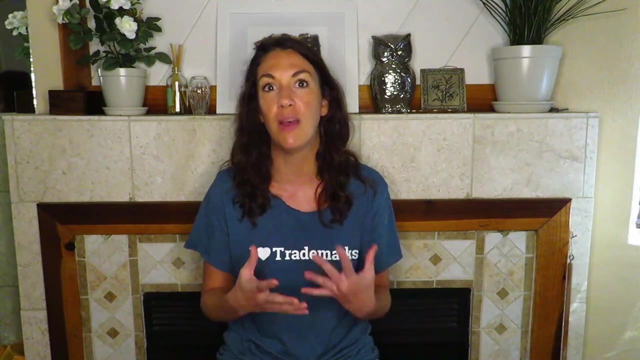 light that you've lied or put inaccurate information on your trademark application initially and so that could be grounds for canceling your trademark altogether or even some other kind of penalties. if you did you know knowingly or if you intentionally put false information or something like that, a lot more issues can come up. but so the point here is a. 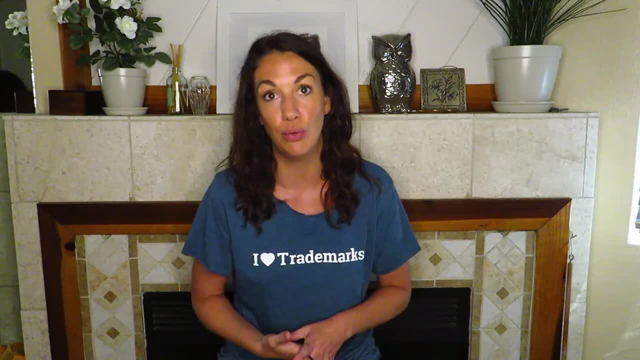 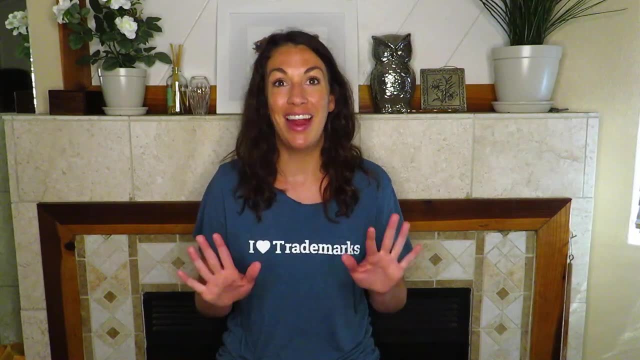 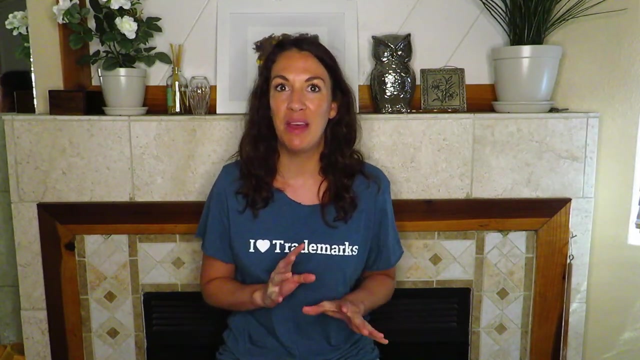 big mistake is not using the right date of first use, because if a issue ever arises, that's going to be the date that we're focusing on, so we want to make sure it's accurate. and then, finally, a pretty- I mean not a huge mistake, but a common mistake that I see happening- is failing to miss. 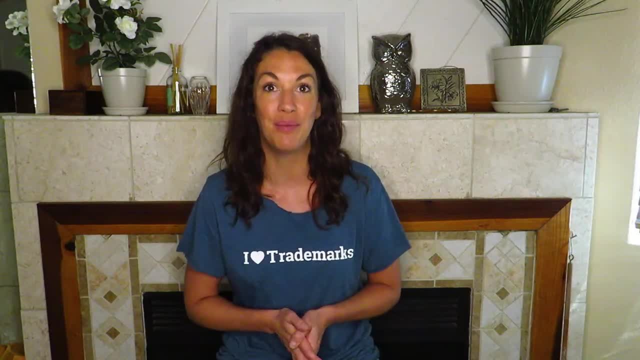 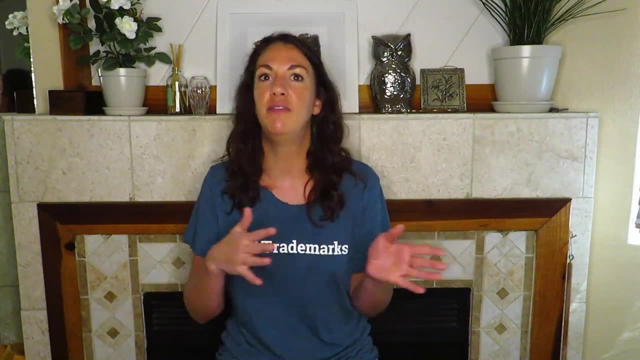 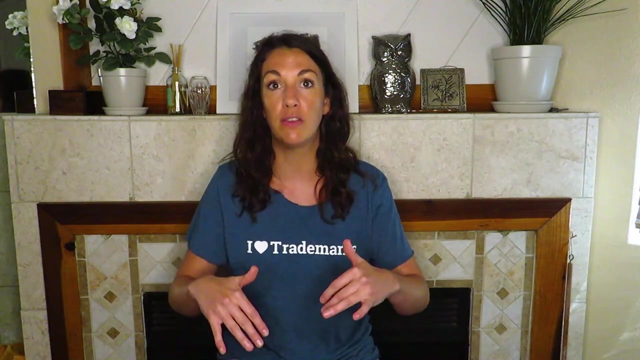 requirements for the TEAS plus application. so when we're filing a trademark application, there are a few different types of applications that we can use and they vary in fees. the cheapest one is the TEAS plus application, which gives you the lowest filing fee in order to use that. 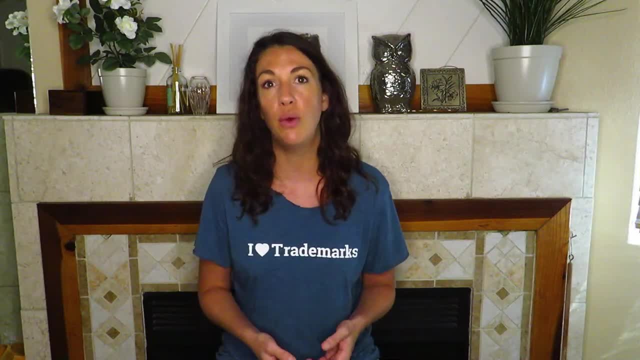 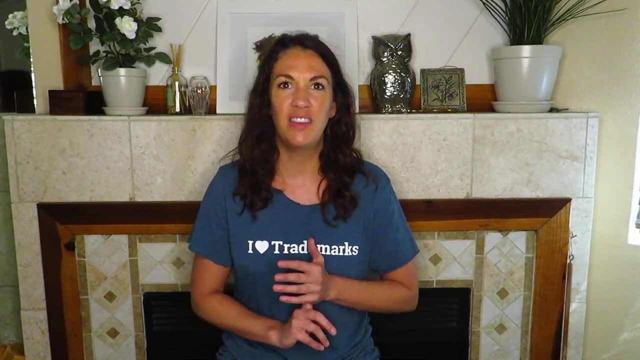 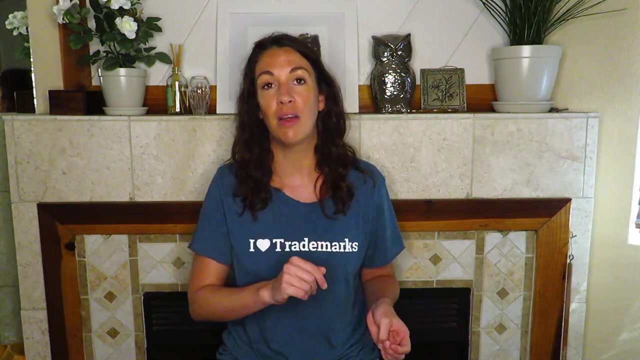 application and take advantage of that low filing fee. the USPTO has a few requirements for what qualifies us to use that application. one of the big ones is agreeing to correspond over email with the USPTO. so if you forget to check that box on the application that says i agree to correspond with. 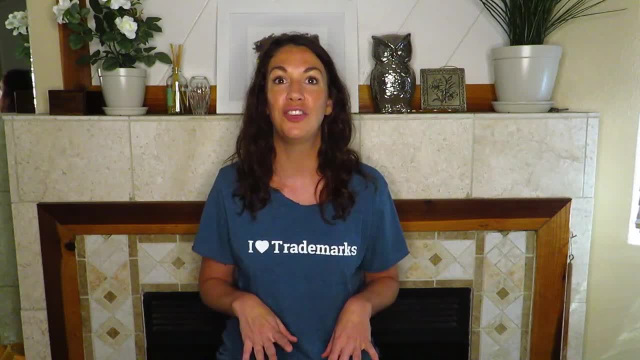 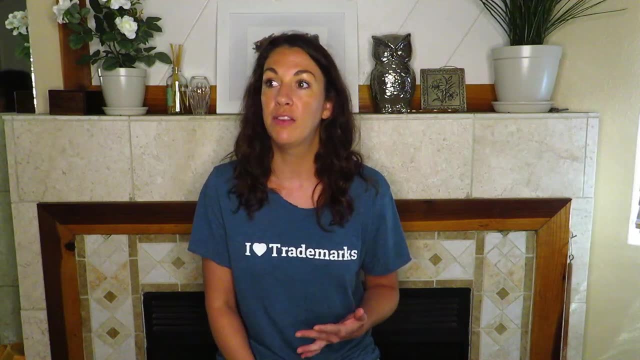 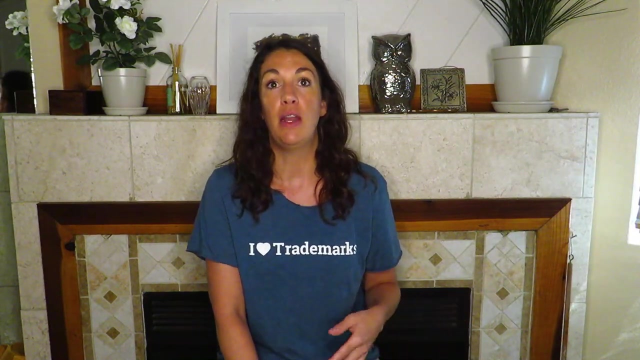 the examining attorney via email, then you're going to lose that eligibility for that reduced fee or that reduced filing fee with that application. other requirements are if: if your trademark includes a person's name or likeness, then you have to give the consent of that person. so let's say, my name, Aiden, was included in that process. if I want to be able to serve on this,